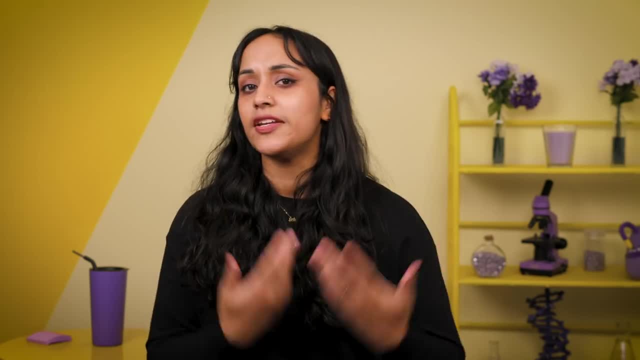 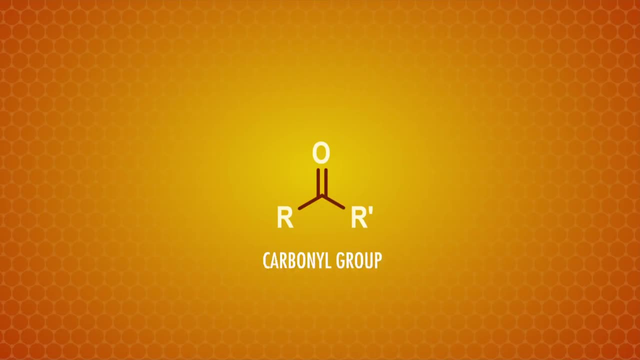 but with more detail. If you're diving in here, or even if it's just been a while since you watched them, you may want to check out some of these episodes as a refresher. We're going to be dealing with a lot of carbonyls. 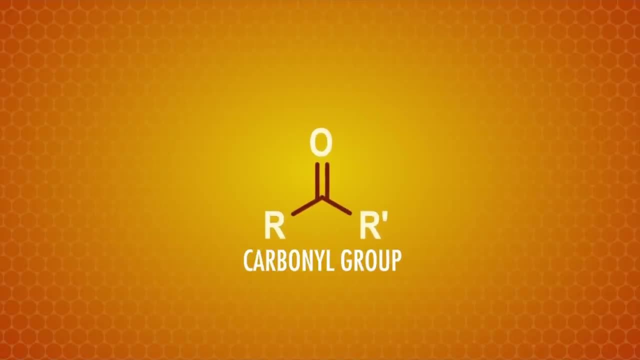 a carbon attached to an oxygen with a double bond like this, The central carbon in this group is called the carbonyl carbon. When it's at the end of a chain attached to a carbon group and a hydrogen, we're dealing with an aldehyde. 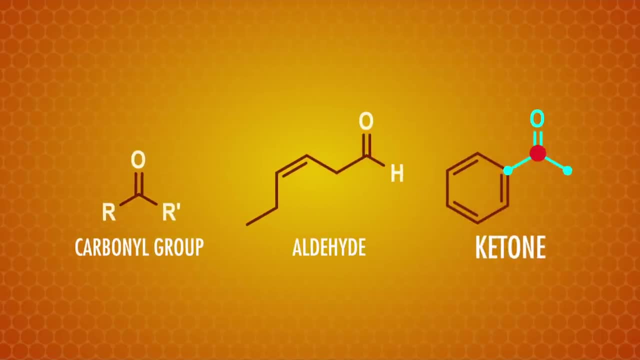 Or when the carbonyl carbon is attached to two carbon groups. it's a ketone. To name an aldehyde, you just take the standard name for the carbon chain and pop an "-al-" for aldehydes on the end. 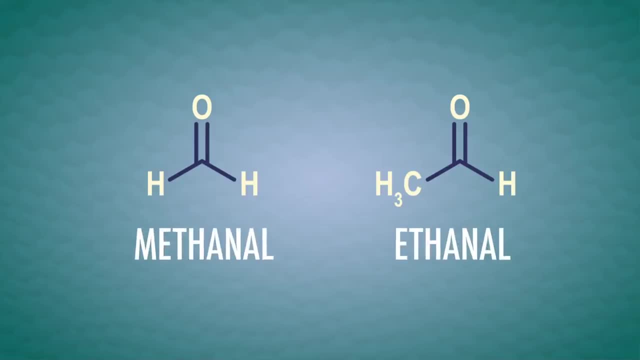 For example, these aldehydes are methanol and ethanol, But these substances have been used by chemists for ages. In fact, ethanol was first discovered nearly 250 years ago. so they have these old common names that you have to learn if you want to talk the talk. 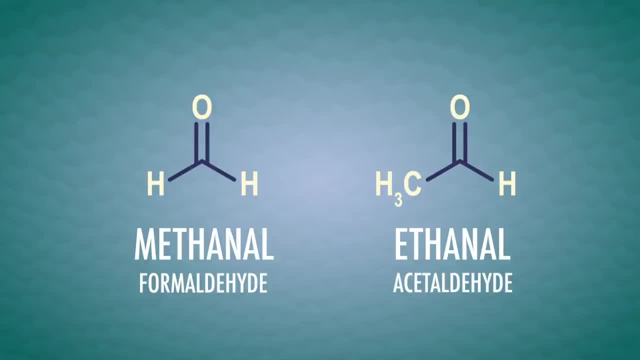 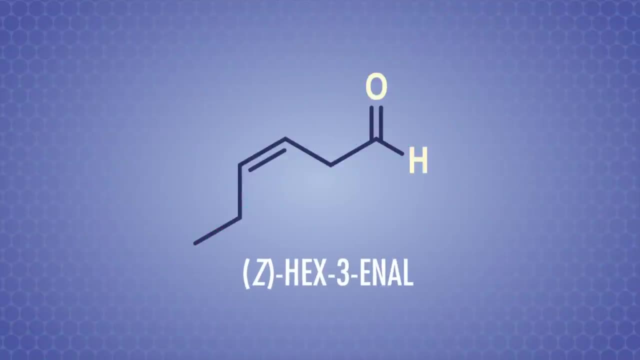 Thankfully, many of them are straightforward and just end in aldehyde like acetaldehyde and formaldehyde. Other aldehydes go by their IUPAC names, For example Z-hex-3-enal. smells of freshly cut grass and leaves. 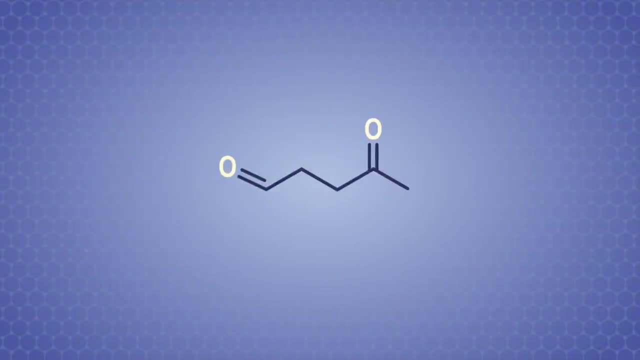 and is an attractant for lots of insects. And even though 4-oxopentanil has both a ketone and an aldehyde, the aldehyde takes priority in nomenclature and is designated position 1. We count along the carbon chain and stick on the prefix. oxo to indicate that the ketone is on carbon 4.. Which brings us to ketones, which all have own on the end, so they're relatively easy to spot. Some rely on IUPAC names, which are not as fun to say. 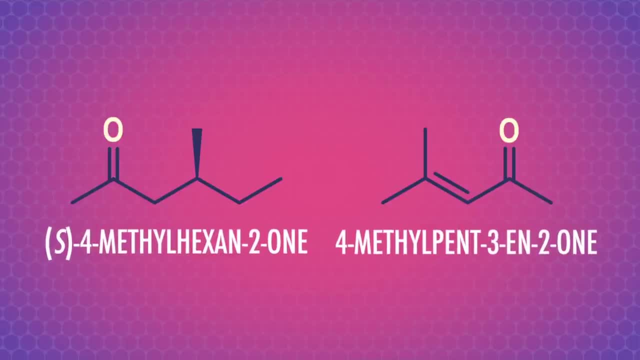 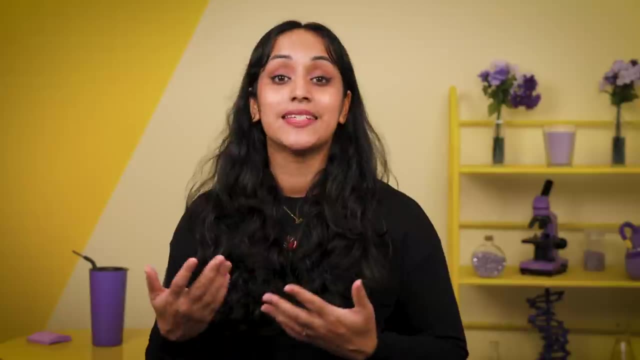 so we'll just put them on the screen. That's video magic. And others have common names such as acetone and acetophenone. Now that we've practiced naming aldehydes and ketones, we can get into making them. 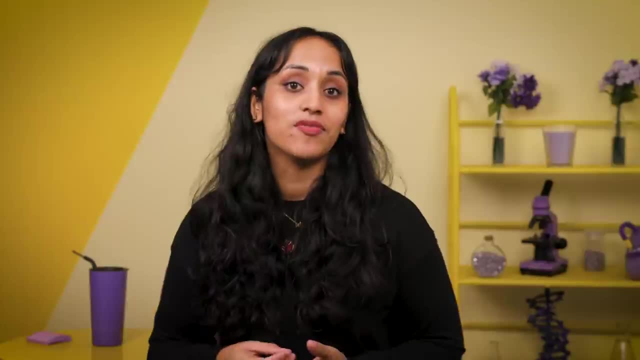 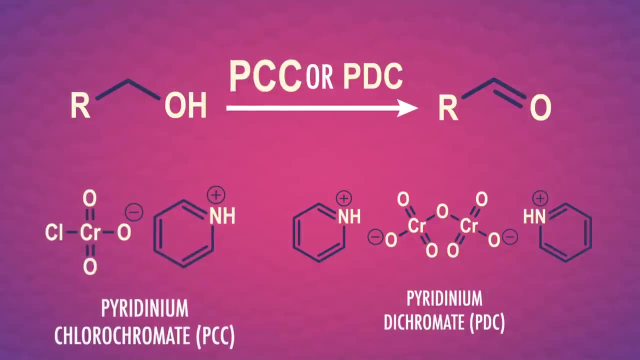 We've actually seen most of these methods already, so they'll hopefully sound familiar. For example, in episode 24, we learned that primary alcohols can be oxidized to form aldehydes. With a weaker oxidizing agent, such as pyridinium chlorochromate, the reaction stops at the aldehyde. Using strong oxidizing agents like chromic acid or even chromate salts is trickier, though. Even though the reaction goes through an aldehyde intermediate, powerful oxidizing agents can produce carboxylic acids To get ketones. you can oxidize secondary alcohols with strong oxidizing agents like chromium 6.. 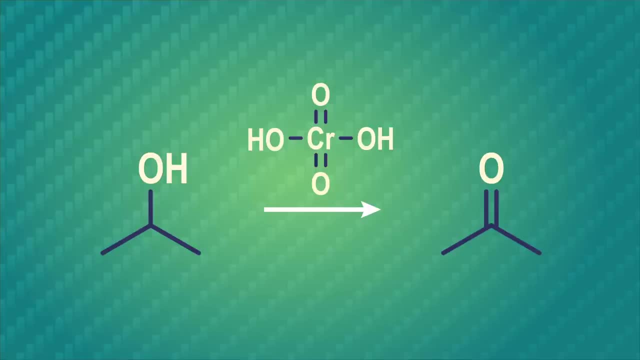 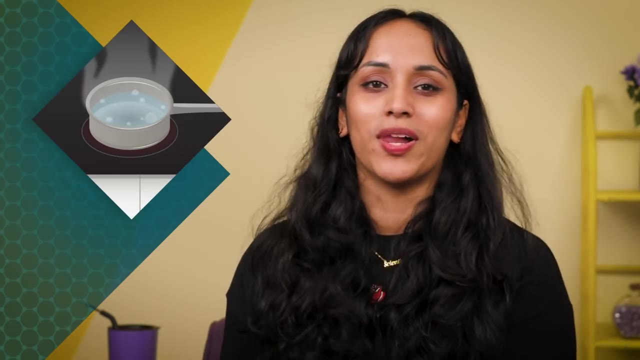 We don't need to be so careful picking our reactants with secondary alcohols, because they can only oxidize to the ketone. These oxidation reactions are often heated, But if you've ever forgotten about boiling water on the stove, you may have come back to a pot with little or no liquid in it. 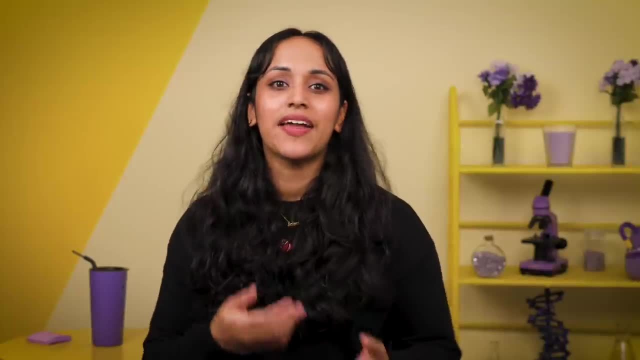 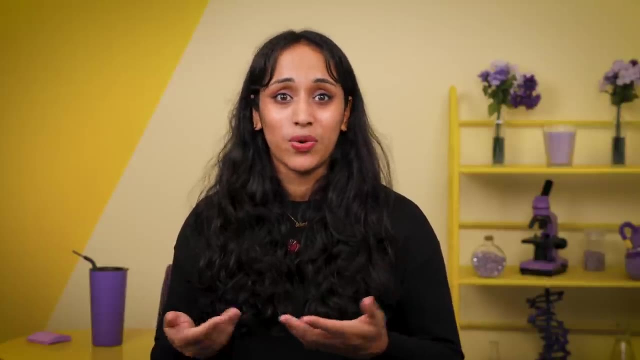 Just like pasta won't soften in a waterless pot, we can't let all the liquid solvent evaporate from our reaction. Most reactions require solvent and the reactants can even burn up if we keep heating without solvent. This is where a technique called reflux comes in. 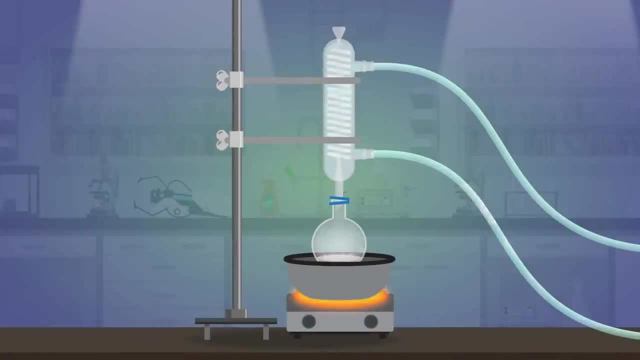 which involves heating a chemical mixture while cooling any evaporated solvent so that it condenses back into the liquid. That way we don't lose anything, even after heating for a long time. No forgotten stovetop accidents. here You can remember it like acid reflux. 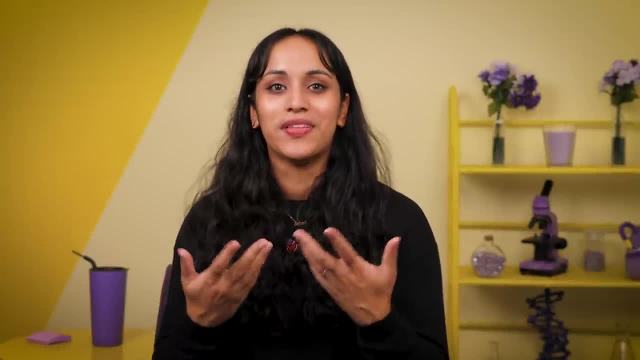 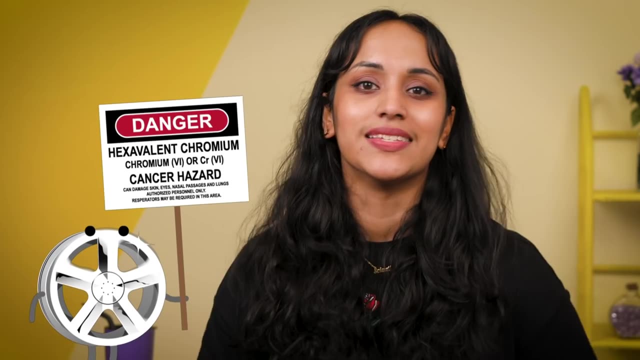 that burning sensation when stomach acid bubbles up towards your throat and then rejoins your digestive juices. The thing is, even though chromium 6 is a useful oxidizing agent, it's unpleasant stuff: Cancer, respiratory problems, kidney disease, you name it. 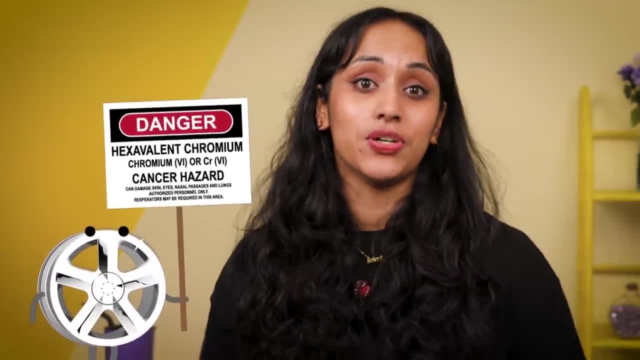 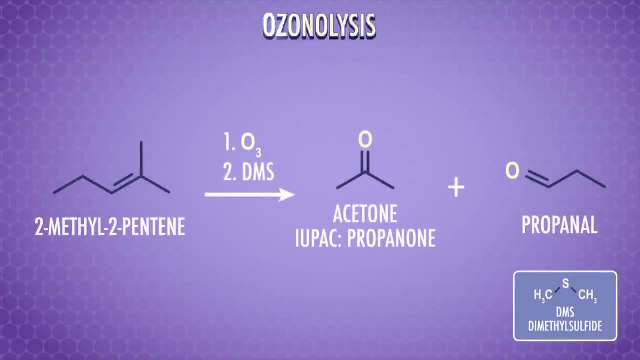 So we can use different oxidizing agents to make aldehydes and ketones too. One option is ozone, O3, which is both higher-yielding and kinder to the environment. The reaction is called osinosis, which we talked about in episode 17 with redox reactions. 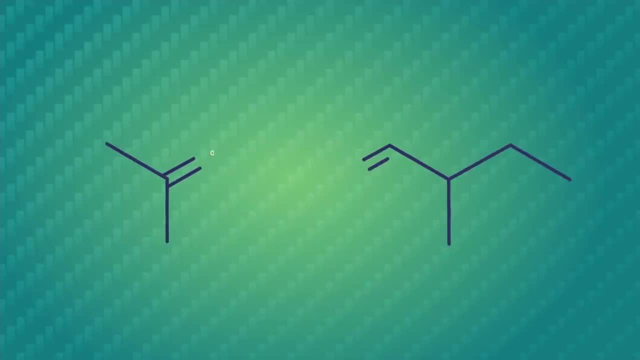 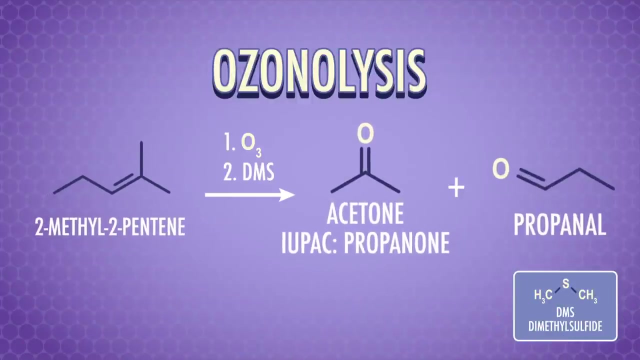 In this reaction we break the double bond of an alkene and form a carbonyl on each side of the carbons involved. For example, osinosis with 2-methyl-2-pentene gives us both acetone and propanol. 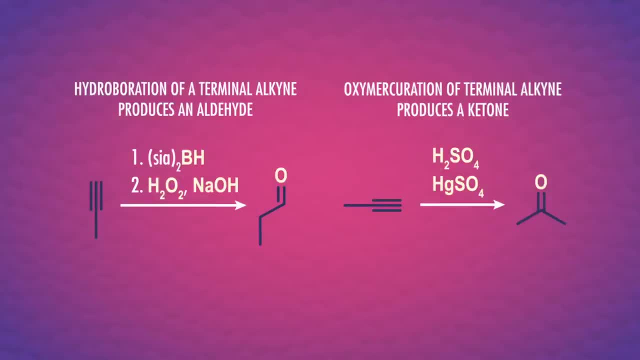 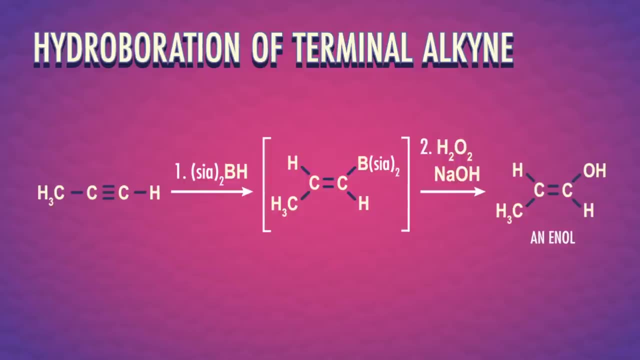 If we start with a triple-bonded alkyne, we can also make our way to aldehydes and ketones. We have hydroboration, which is anti-Markovnikov addition. In episode 18, we showed BH3 for simplicity. 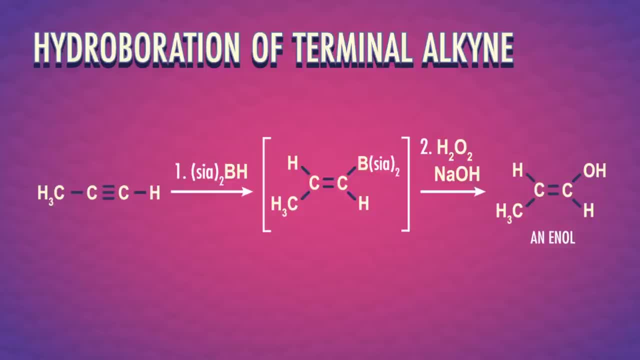 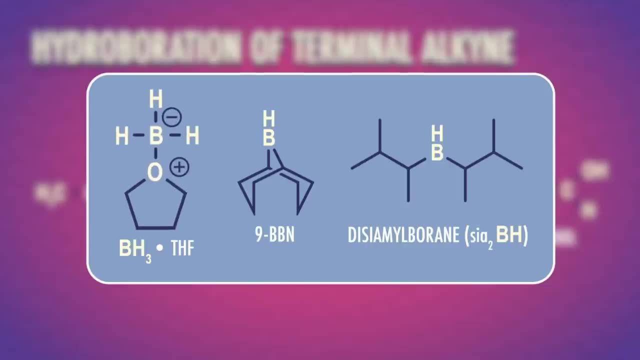 but BH3 doesn't actually exist in that body. There are more common, even bulkier reactants we can use to get really good anti-Markovnikov selectivity, like borane, THF, a cool double ring structure called 9-BBN- and disamylborane. 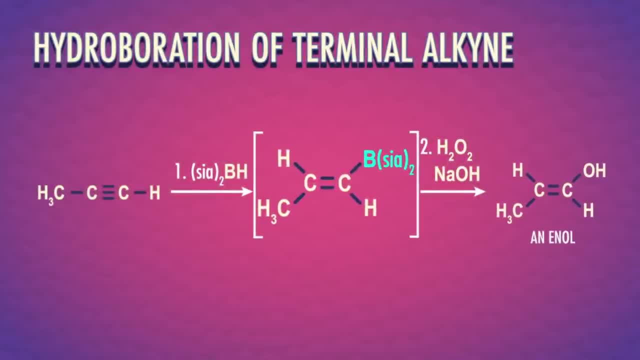 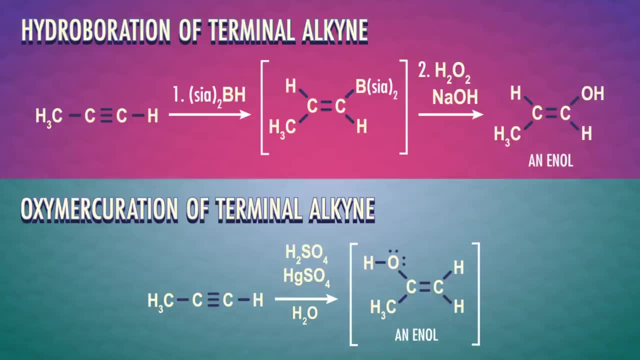 In hydroboration we form the less-substituted enol thanks to the borane intermediate that forms from the bulky boron reagent. On the other hand, oxymercuration is Markovnikov addition and gives us the more-substituted alcohol. 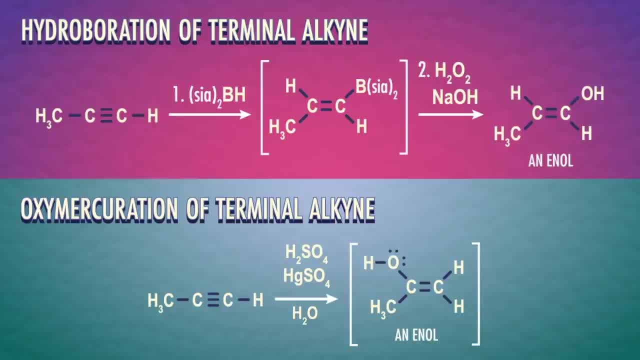 But we're not done yet. The enols that form from each of these reactions aren't very stable, and they exist in equilibrium with more stable carbonyl or keto forms. This balance ultimately gives us aldehydes, or ketones, from these reactions. 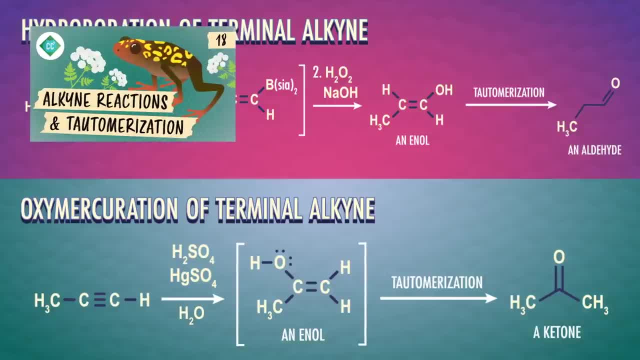 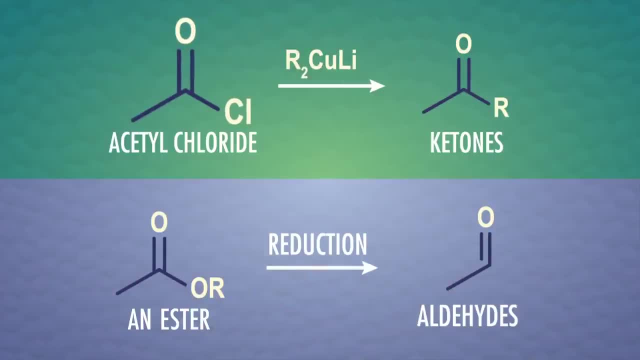 We covered this mechanism in a lot of detail in episode 18, if you want to check back, There are a few more options that we haven't learned yet, but here's a quick preview. Acid chlorides can react with organocopper compounds to give us ketones. 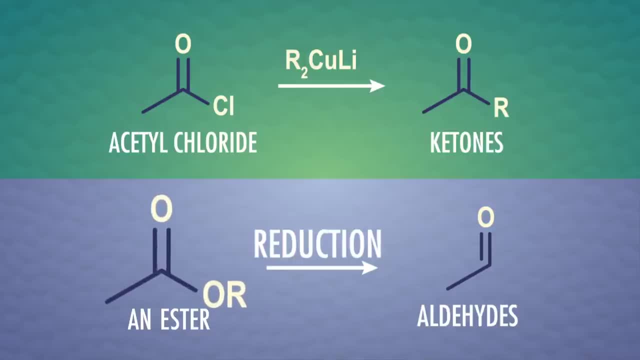 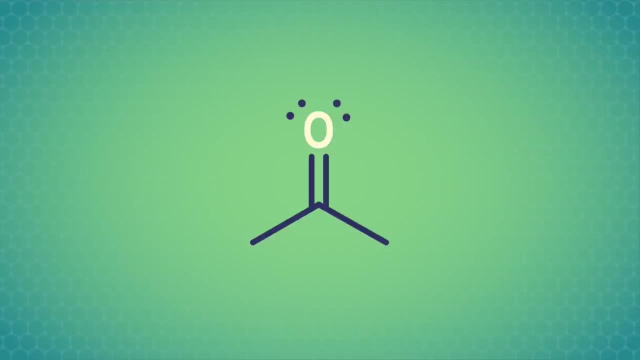 and using special bulky reducing agents on esters can produce aldehydes. Now part of why we care about making aldehydes and ketones is because chemists can judge so many things with them. The carbon-oxygen double bond is polar, so we have a dipole. 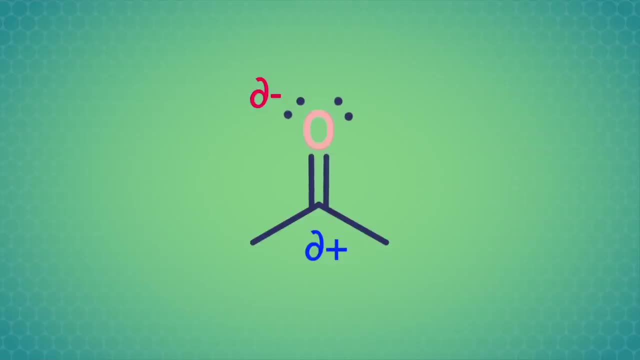 In fact, because the oxygen is so electronegative, we actually end up with dipolar resonance, where in one form the oxygen atom has a negative charge, while a carbonyl carbon has a positive one. All of this means the carbonyl carbon is a prime target for nucleophilic attack. 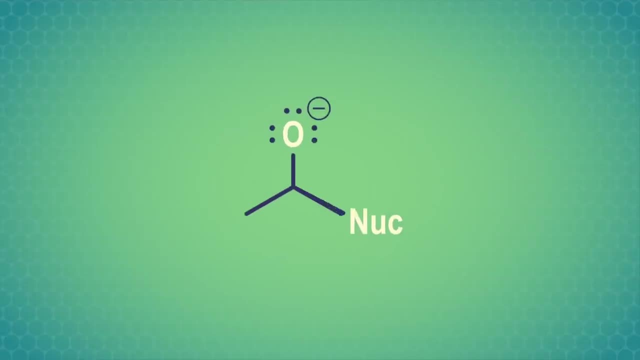 specifically in addition reactions, because there's no leaving group. We end up with an sp3- carbon and electrons pushed onto a negatively charged oxygen which will tend to pick up a proton when we add some water at the end of the reaction and form an OH group. 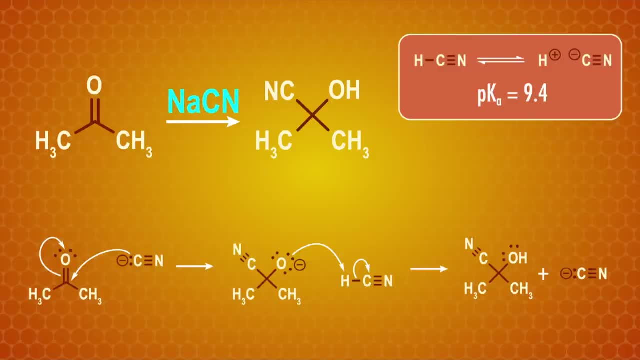 A handy nucleophile we can add to the carbonyl group is a cyanide salt, CN-. This gives us a new functional group in the molecule that we can turn into other things like amines and carboxylic acids. We'll get to know these reactions much later in the series. 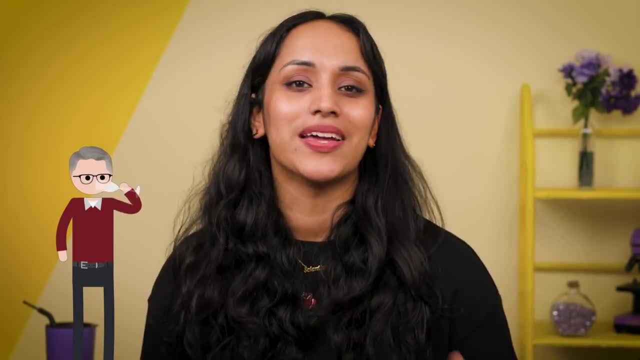 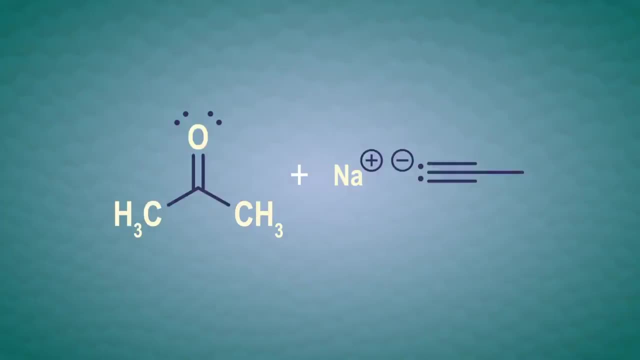 Of course, if you've read any Agatha Christie, you might know that sodium cyanide is one of the most rapidly acting poisons, so double-check your risk assessment for this one A less scary reaction. A less scary reaction from a health and safety point of view. 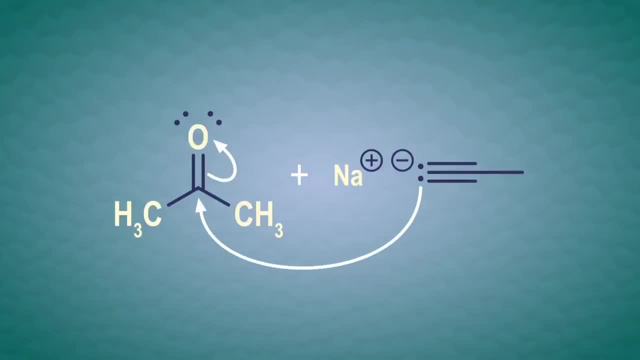 is using an acetylide anion as our nucleophile. The acetylide attacks the carbonyl carbon to ultimately form an alcohol with an alkyne functional group, sometimes called a propyl alcohol. We can also choose hydride anions as our nucleophile. 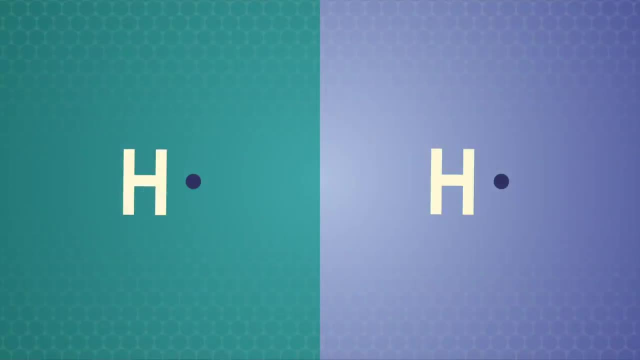 And yes, you heard me correctly. a neutral hydrogen atom often loses its one electron to become H+, but it can also gain an electron to have a pair and form H- Examples of hydride reagents are sodium, sodium borohydride. 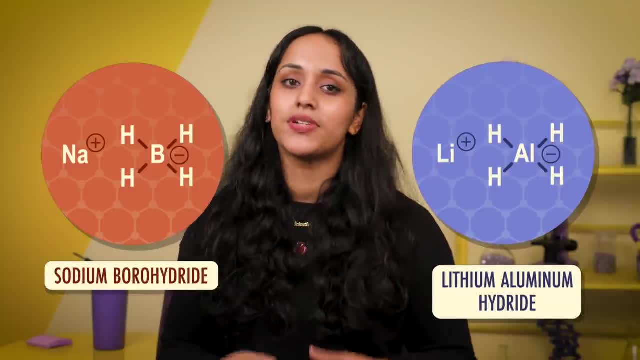 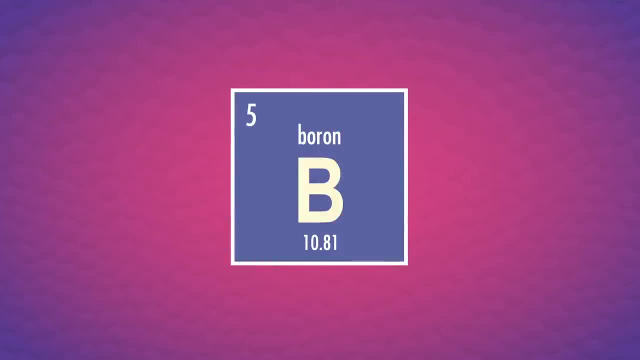 and lithium aluminum hydride. Let's look at the mechanism of this reduction reaction using sodium borohydride. Boron is an electropositive atom with only three valence electrons. It doesn't follow the octet rule and tends to form neutral compounds with three covalent bonds. 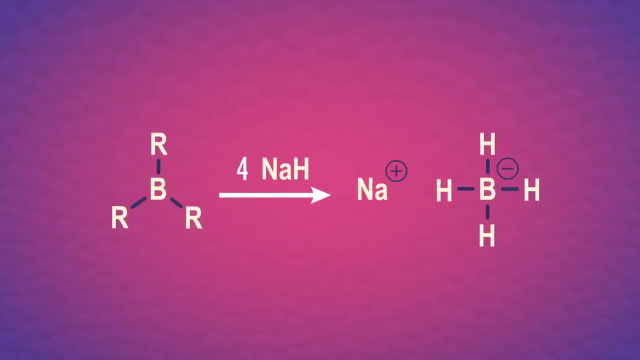 But it will accept electrons into its empty p-orbital and form a borohydride anion- BH4-. When a borohydride anion attacks the carbonyl group in an aldehyde or ketone, both the electrons in that fourth BH. 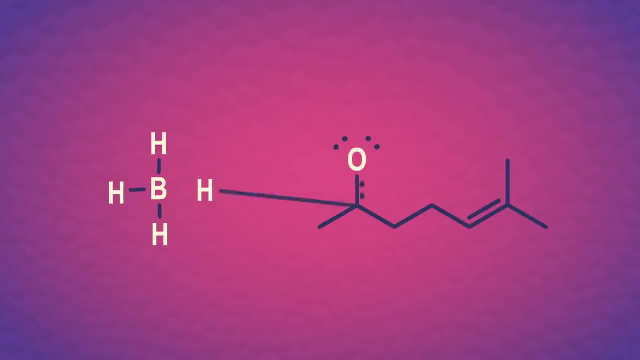 go with the hydrogen. So this reaction results in neutral BH3 and an alcohol anion. This alkoxide can then react with the water in the reaction to form an alcohol, Specifically a primary alcohol if we had an aldehyde and a secondary alcohol if we had a ketone. 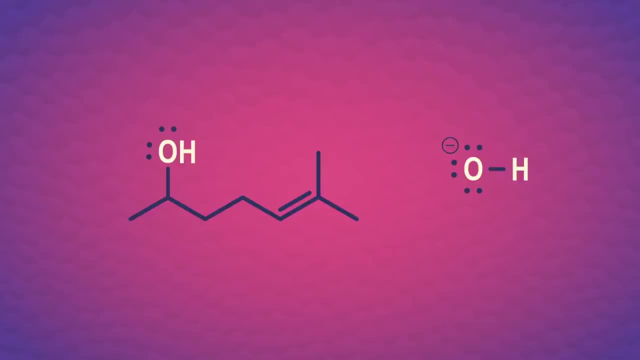 Notice, the double bond in the molecule doesn't react and the hydride anion only attacks at the electropositive carbonyl carbon. And since aldehydes and ketones have trigonal planar molecular geometry, the hydride can attack one electron at a time. 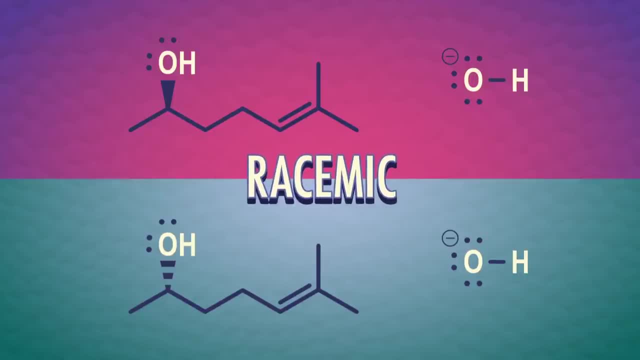 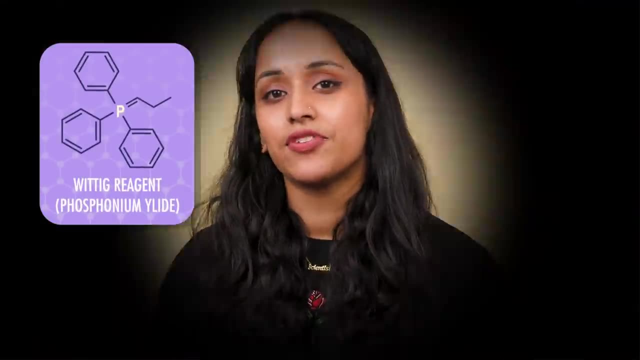 It can attack one side or the other and we get a racemic mixture at a chiral carbon. One last reagent that deserves a mention is the Wittig reagent, aka phosphonium illid. It's named after George Wittig. who won the Chemistry Nobel Prize for his work in 1979.. An illid- and yes, that's spelled Y-L-I-D-E, because English is annoying sometimes- is a molecule with adjacent atoms that have opposite formal charges, Specifically a negatively charged carbanion attached to an atom. 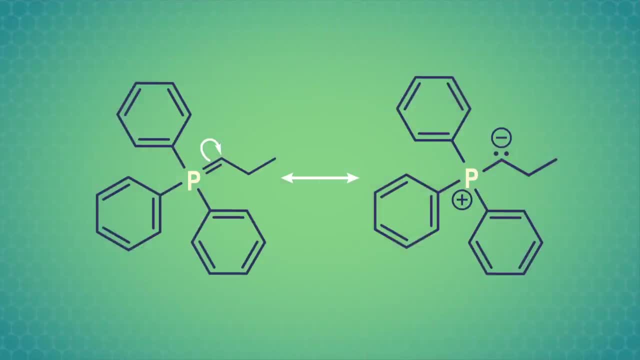 with a positive charge In the Wittig reagent. the positively charged atom is phosphorus in a compound known as phosphorine. This is another example of a resonance structure. So when we react an aldehyde or a ketone via the Wittig reaction, 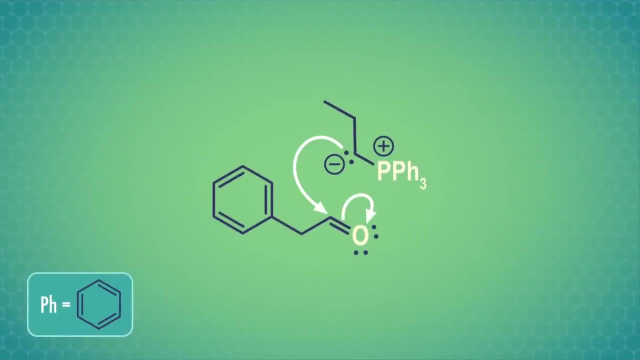 the mechanism begins when the nucleophilic carbanion of the illid attacks the electropositive carbonyl carbon. similar to these other reactions we've been doing. This makes a zwitterion a molecule containing atoms with positive and negative formal charges that are not adjacent. 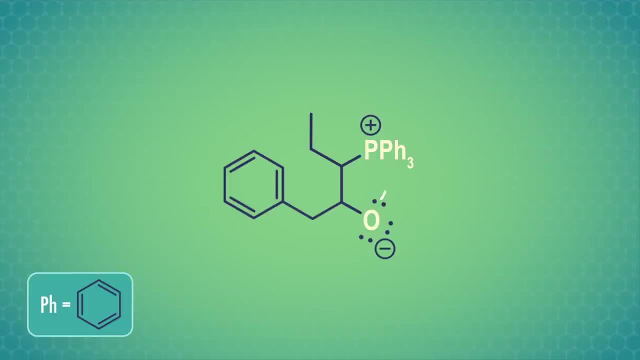 so it's slightly different from an illid. In this case, the negatively charged oxygen of our zwitterion quickly reacts with the positively charged phosphorus to form a four-membered ring species called a 1,2-oxaphosphatane. 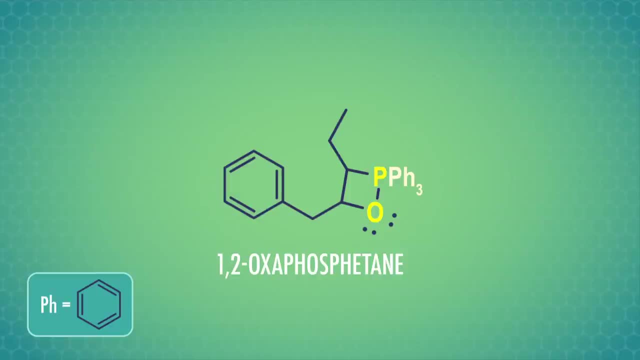 The 1,2 in the name tells us, the oxygen and phosphorus are next to each other at the 1 and 2 positions of the four-membered ring. The small ring is super unstable, while phosphorus-oxygen double bonds are very stable. 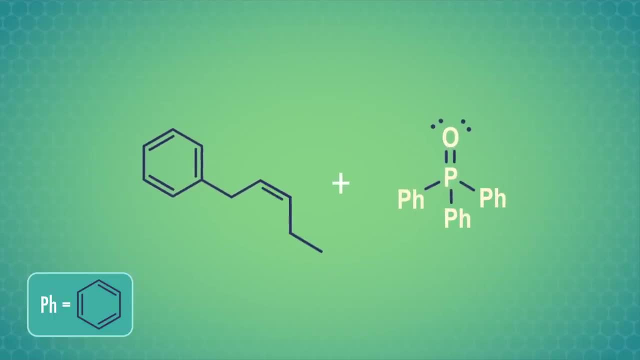 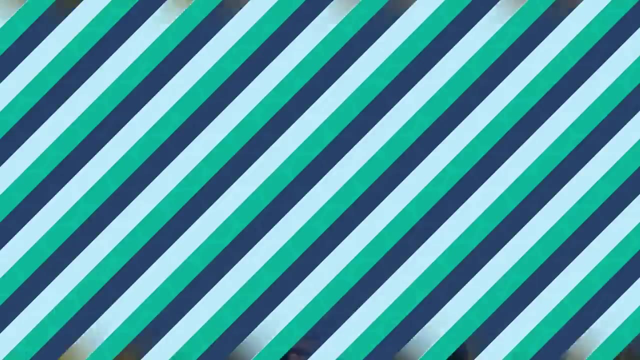 so the oxaphosphatane collapses to form an alkene and triphenylphosphenate or phosphine oxide. This process is so fast we often represent it as one step with two arrows. And, by the way, this reaction only worked with a primary illid. 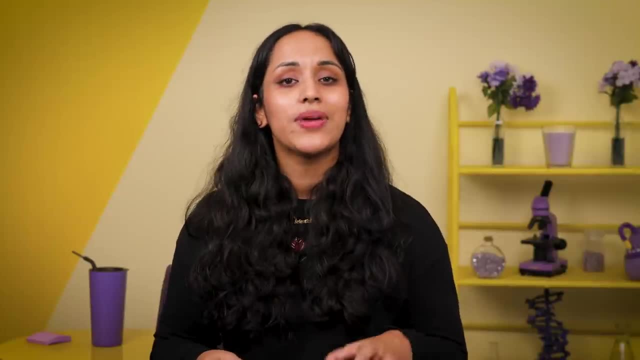 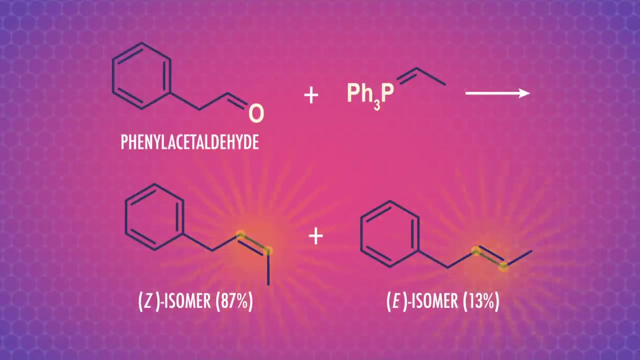 If we had two alkyl groups on the negatively charged carbon. the reactant is too chunky and the reaction doesn't work. The Wittig reaction is another carbon-carbon bond-making reaction, and chemists really love those. Specifically, we form a Z-alkene as the major product.